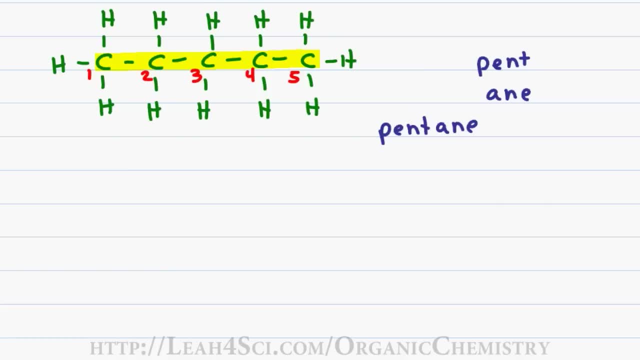 109.5.. This means if your molecule is drawn out more realistically, it'll actually look something like this: Don't let the angles between the carbons fool you. If you can place your highlighter on the first carbon and then trace it all the way to the end of the chain without having 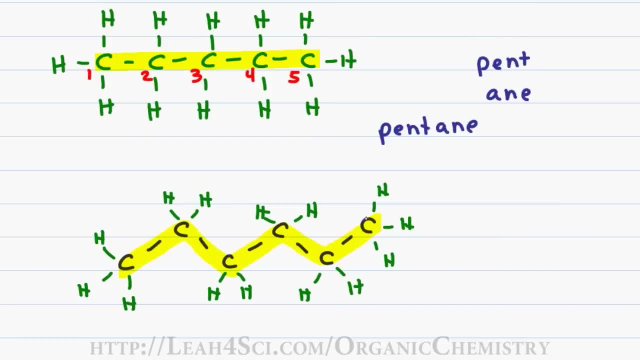 to lift in the middle. this tells you that you have one continuous parent chain. Once again, I can number from either direction and now apply the puzzle pieces. For the first name, I have six carbons, which gives me a first name of hex. I only have single bonds. 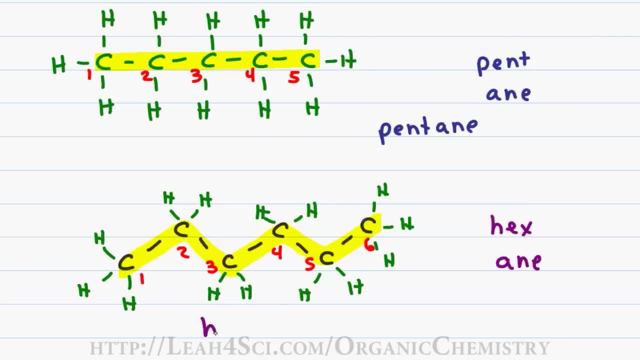 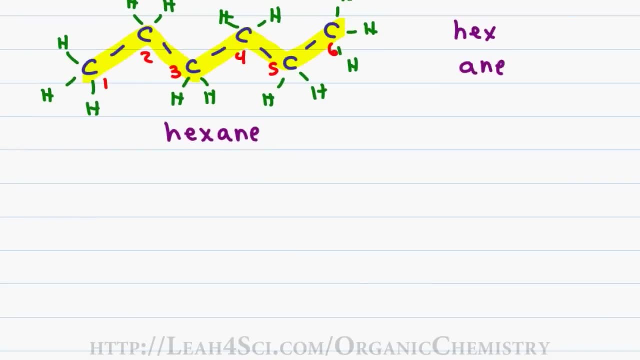 which gives me ane, and that means this molecule is hexane. A faster and simpler way to draw this molecule is by using line structure. I'm going to follow the exact shape of what I have above to represent the six carbons. Recognize that every end and every angle represents another carbon. 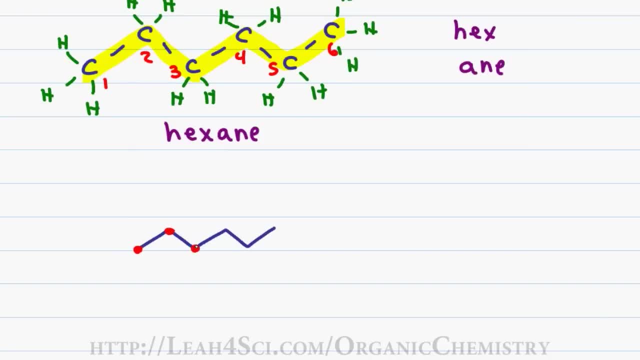 atom and all the hydrogens are invisible and not that important to name it. I approach a molecule in line structure in the same manner where I first highlight the parent chain and then assign numbers to help with the naming, Once again recognize that we have six carbons. 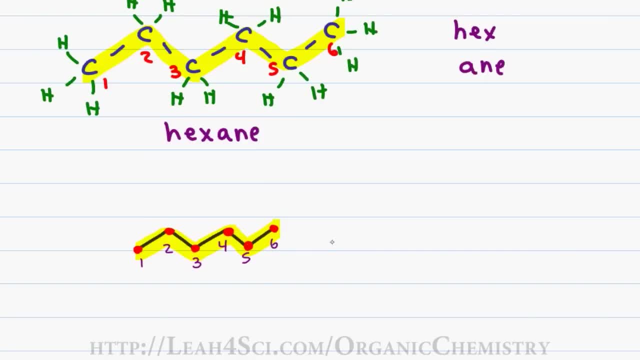 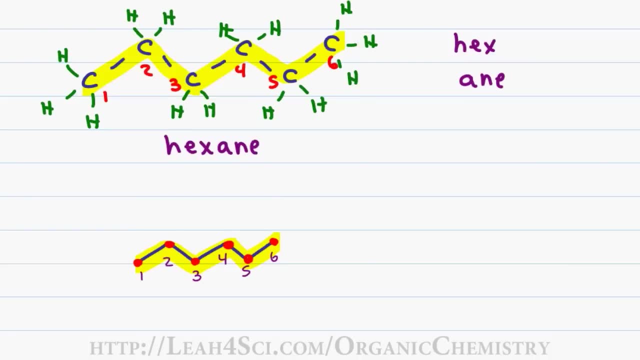 and therefore the molecule hexane. Since carbon to carbon single bonds have the ability to rotate, you can see this molecule represented in a non-linear manner. Looking at the structure I drew here, I still have only six carbons and therefore only hexane. So no matter how, 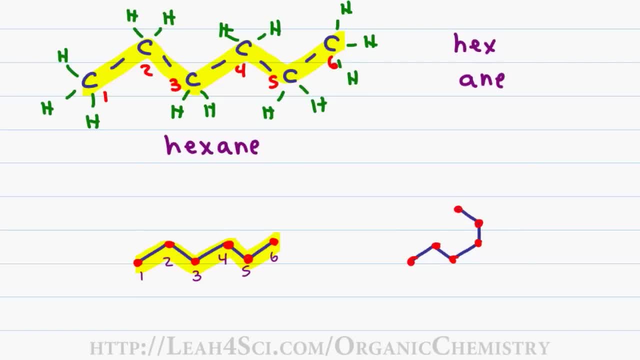 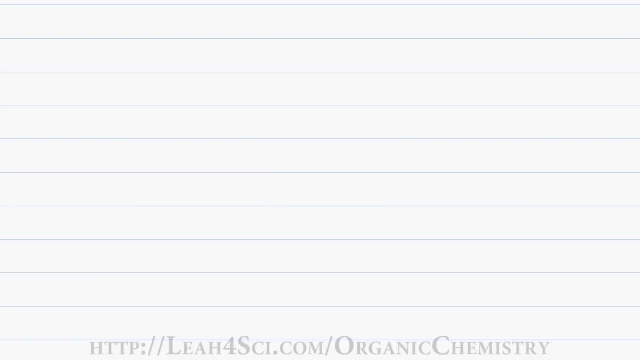 the molecules presented to you. don't let that fool you. Let's look at one last simple example before moving on to branched alkanes, and we'll use this structure as our example. The first thing I want to do is highlight my parent chain. 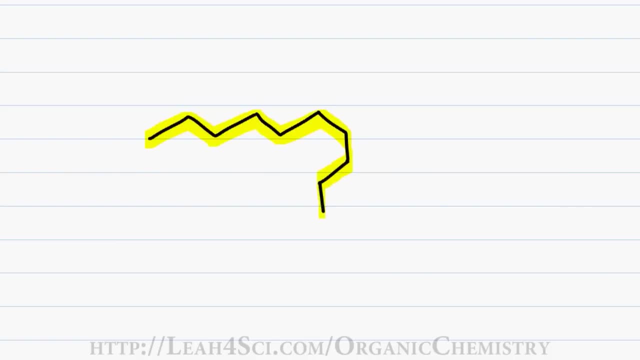 since I don't have to lift the highlighter from beginning to end. that tells me this is one continuous chain. When I number the chain, I get a total of 10, which gives me a first name of Dec. since I only have single bonds, that gives me a last name of Ane and this gives me Decane, If you feel.